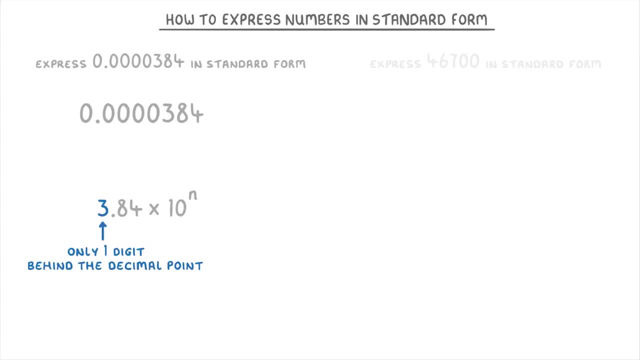 we need to take our original number and count how many places the decimal point needs to move, Which is 1,, 2,, 3,, 4,, 5 places, And this tells us that our power is going to be 5.. 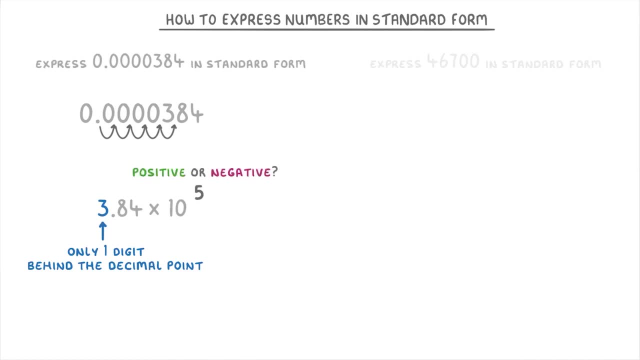 To figure out whether that's a positive or a negative. 5, though we need to look at our original number and see whether it's small or big, Because 0.0000384 is smaller than 3.84, that tells us that our power is going to have to be negative. 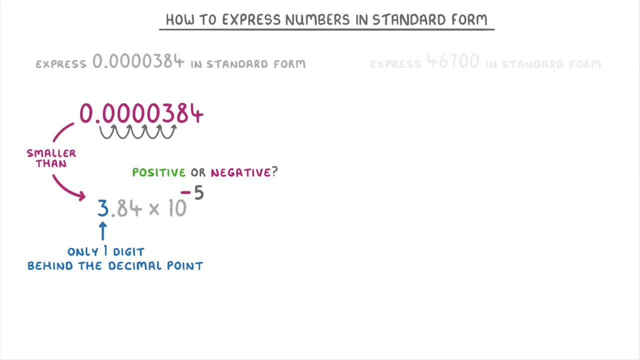 because negative powers make things smaller. So our overall answer is 3.84 times 10 to the power of negative 5.. So our overall answer is 3.84 times 10 to the power of negative 5.. So our overall answer is 3.84 times 10 to the power of negative 5.. 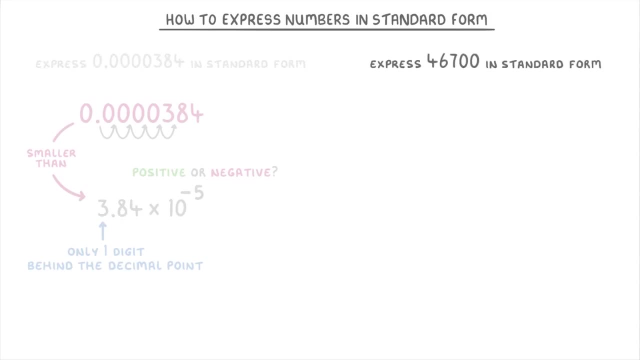 In this next question, we're being asked to express 46,700 in standard form. So, again, the first step is to think about what the front number is going to need to be, Which this time would be 4.67.. 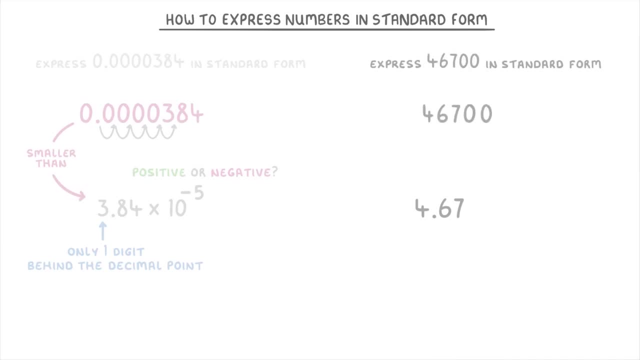 Next we take 46,700, write in the point 0 at the end so that we can work with the decimal point and then count how many places the decimal point needs to be. The decimal point will have to move to get to 4.67, so 1,, 2,, 3,, 4 places. 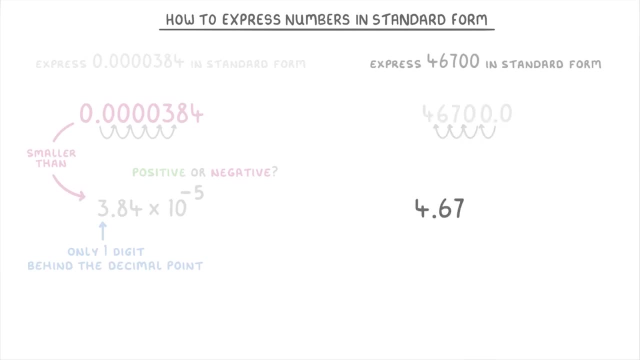 So we now know that our standard form is going to be 4.67 times 10, to the power of either positive 4 or negative 4.. And as 46,700 is bigger than 4.67, it's going to have to be the positive 4.. 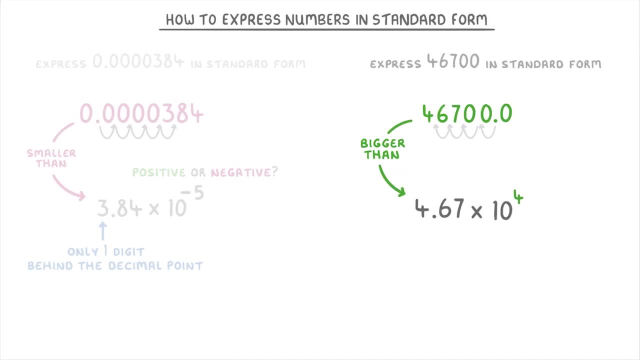 So our final answer is 4.67.. So we now know that our standard form is going to be 4.67 times 10 to the power of positive 4.. Let's have a quick go at two more before we finish. In this first one, we need to convert 0.0029.. 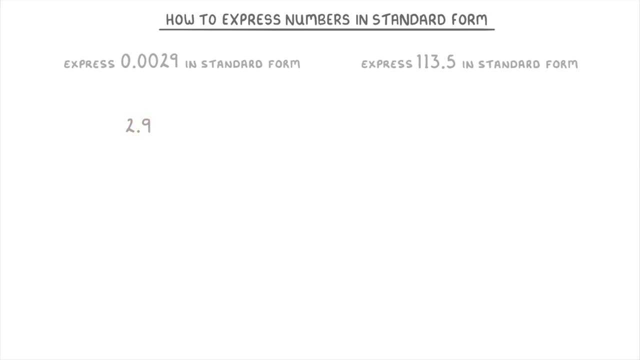 So we write out 2.9 as our front number And then, using little arrows, we can see that the decimal place needs to move 1,, 2,, 3 places, So we can add times 10 to the power of 3..